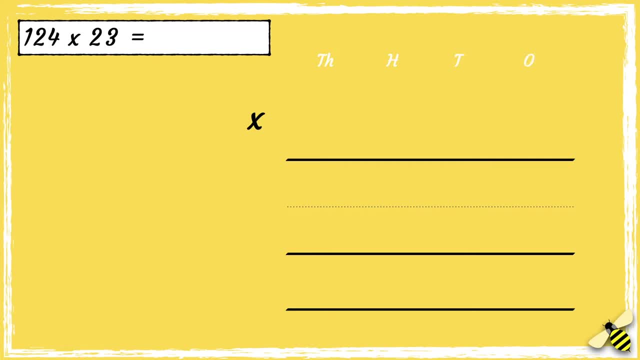 ones. One hundred and twenty-four has one hundred two tens and four ones. Twenty-three has two tens and three ones. So now that we're set up we're ready to multiply. So first we'll multiply three by four. Three times four is twelve. We can drop the one ten below. 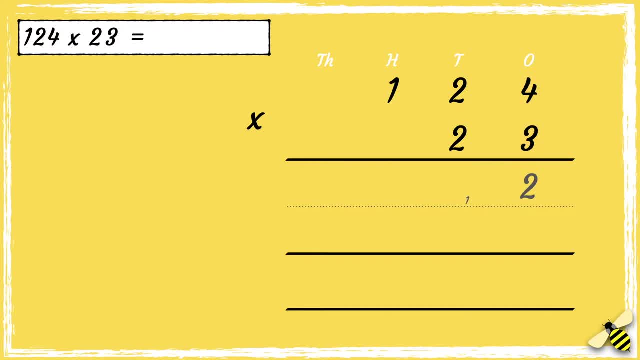 in the tens column. Then we can multiply three by two tens. So three times two is six, and then add the extra one, so it's seven. So now we need to multiply three by one hundred. Three times one is three, So now we need to multiply two. 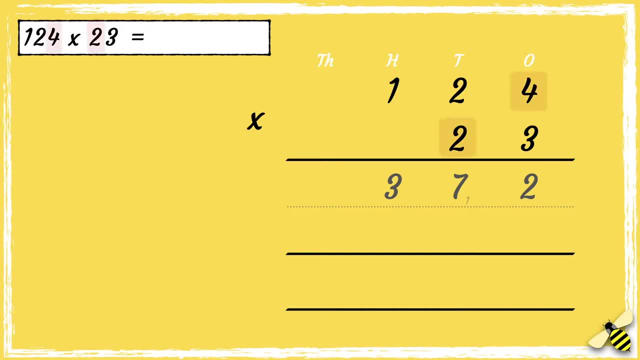 tens by four. As we're multiplying the number by two tens, we need to put zero as a placeholder in the ones column. So now that we've got zero as our placeholder, we can multiply two tens by four. Two times four is eight. 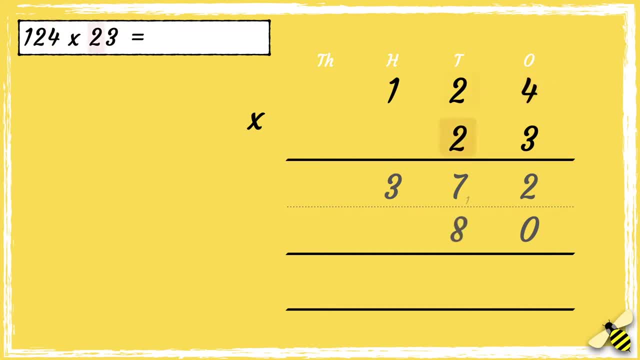 Then we can work out two tens multiplied by two tens. Two times two is four. Then we need to work out two tens multiplied by one hundred. Two times one is two. The next step is to add the two answers together. So two adds zero is two. Seven adds eight. 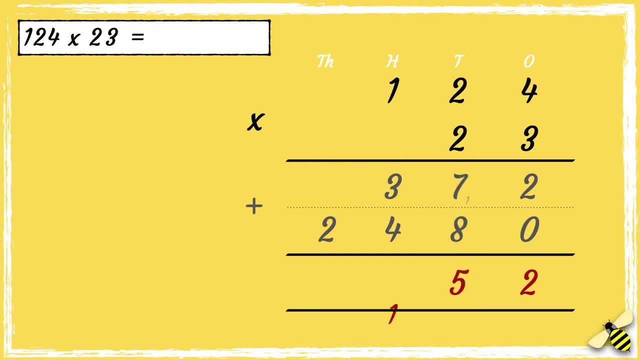 is fifteen. We can carry the ten tens over to the hundreds column to make one hundred. Then three add four add one is eight, And then two add nothing is two. So the answer is two thousand eight hundred and fifty-two. Let's have a look at another example: Two hundred and thirty-seven multiplied by thirty-five. 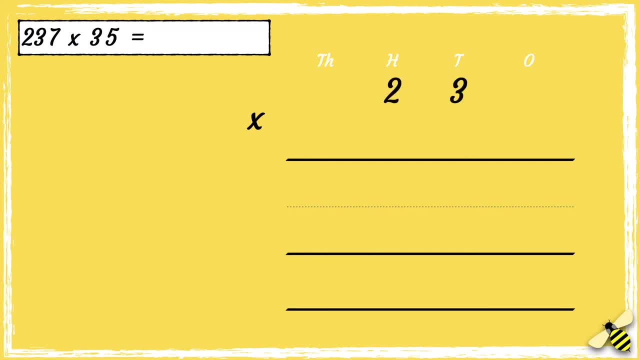 Two hundred and thirty-seven has two hundreds, three tens and seven ones. Thirty-five is three tens and five ones. So now that we're set up we're ready to multiply. So first we'll multiply five by seven. Five times seven is thirty-five. We can drop the three tens below in the tens column Then. 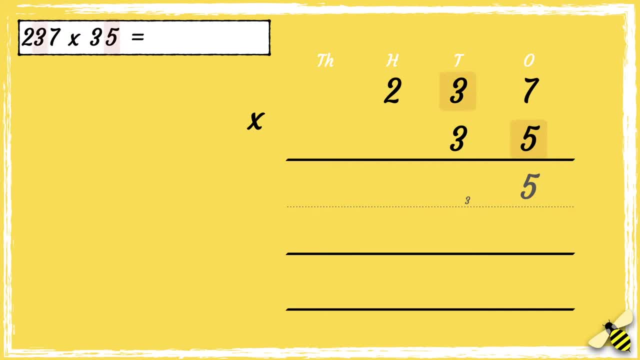 we can multiply five by three tens, So three times five is fifteen, and then add the extra three is eighteen. We can drop the one below in the hundreds column. So now we need to multiply five by two hundreds. So two times five is ten. add one more eleven. 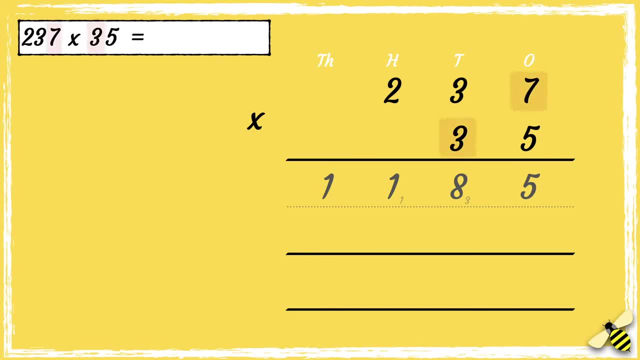 So now we need to multiply three tens by seven. As we're multiplying the number by three tens, we need to use zero as a placeholder in the ones column. So now that we have zero as our placeholder, we can multiply three tens by seven. Three times seven is twenty-one. We. 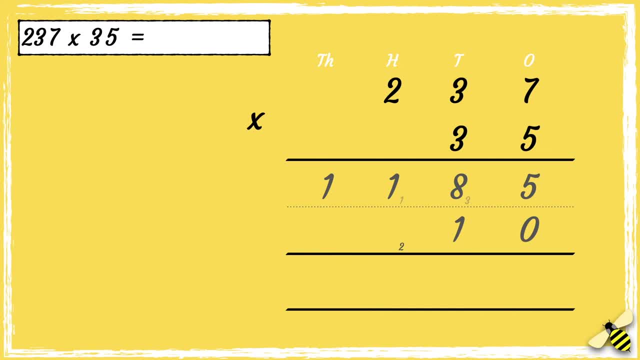 can drop the two below in the hundreds column, Then we can work out three tens multiplied by three tens. Three times three is nine and then add the extra two is eleven. We can drop the one down in the thousands column. Then we need to work out three tens multiplied by two hundreds. Three times two is six and 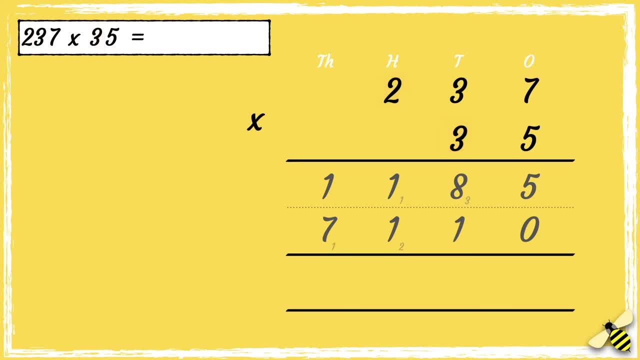 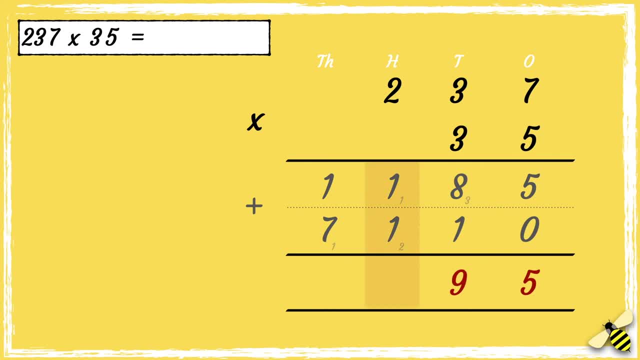 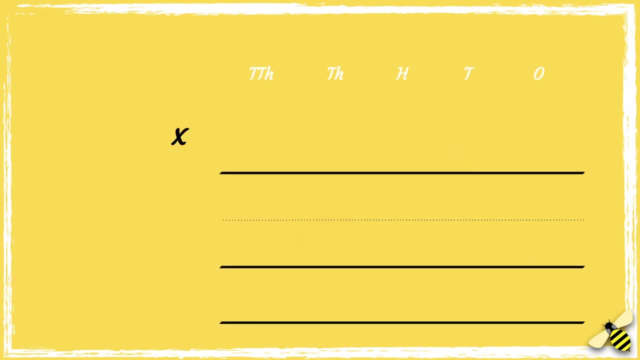 Eight add one is nine, Then one add one is two, And then seven add one is eight. Let's have a look at one more example. Four hundred and sixty-one multiplied by thirty-two, Four hundred and sixty-one has four hundreds, six tens and one one. 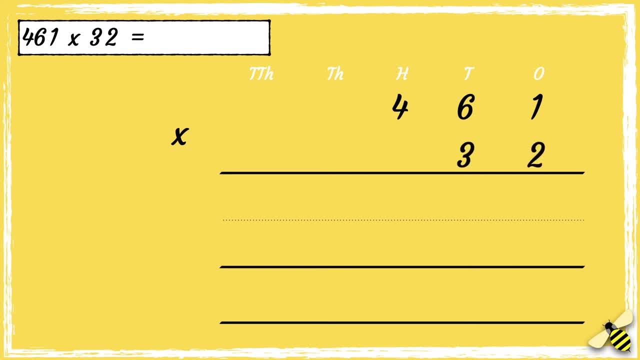 Thirty-two has three tens and two ones. So now that we're set up we're ready to multiply. So first we'll multiply two by one. Two times one is two. Then we can multiply two by six tens. So two times six is twelve. 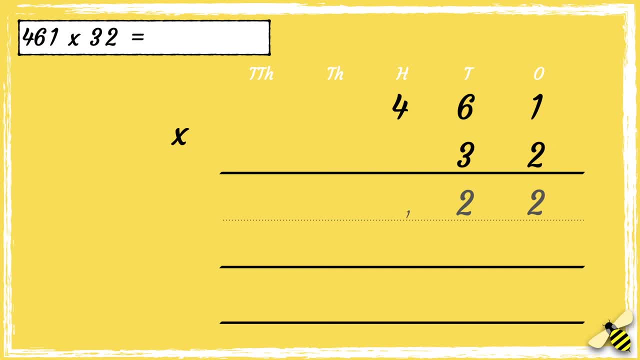